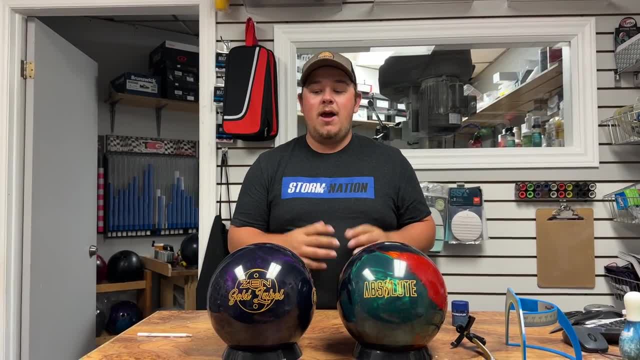 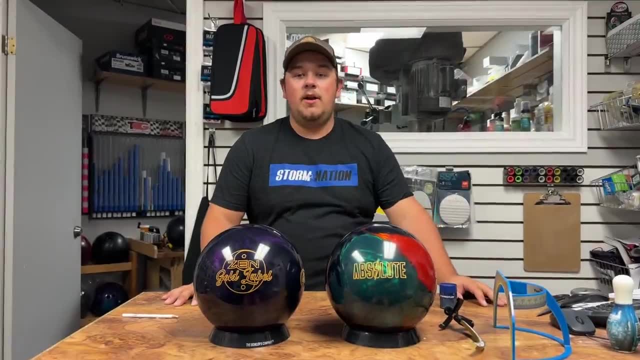 Alright, how's it going, everybody? Today we're going to be doing a video on how to lay out a bowling ball. Stay tuned, Alright. so, like I said in the little intro, there we're going to be doing a video on how to lay out bowling balls. 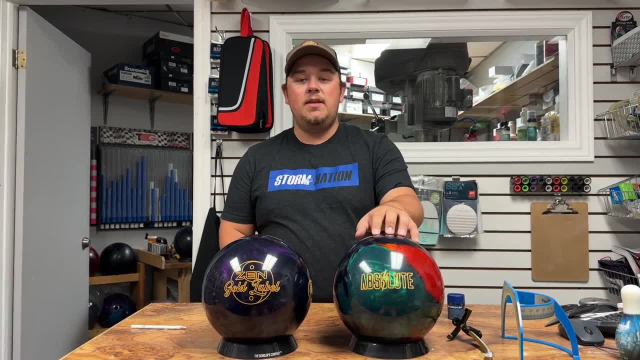 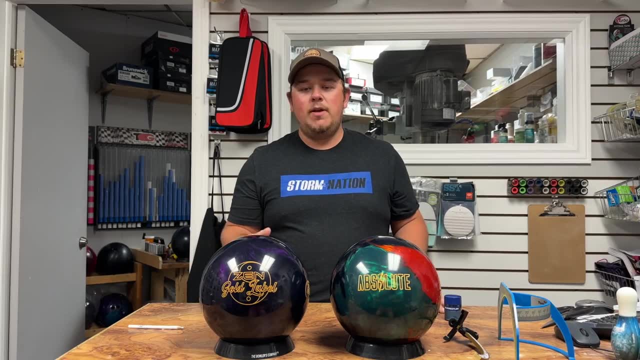 We've got two different bowling balls to lay out today. One is the Storm Absolute, One is the 900 Global Zen Gold Label, And I chose these ones for a couple different reasons. I'm going to show you the importance of the PAP. 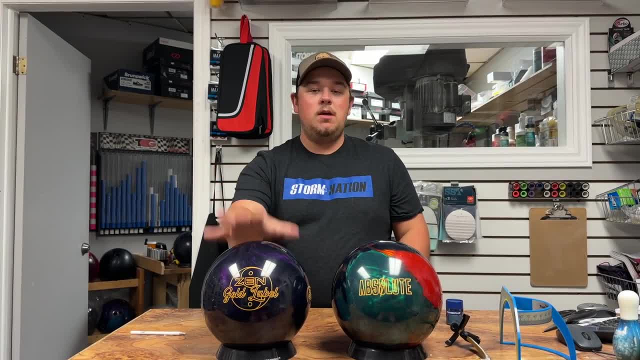 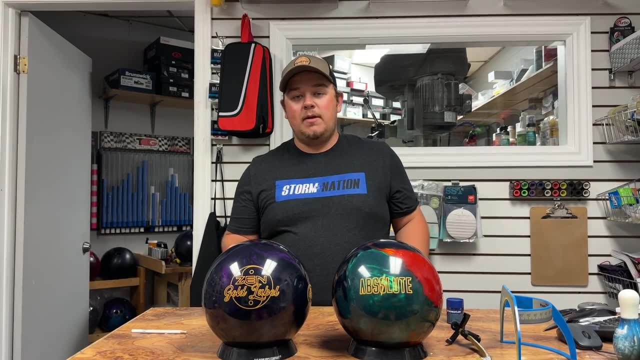 So I'm going to be using one PAP on the Absolute, one PAP on the Gold Label And we're going to be doing the exact same layout: a 5x4x3.. We'll talk a little bit about what those numbers mean in a minute there. 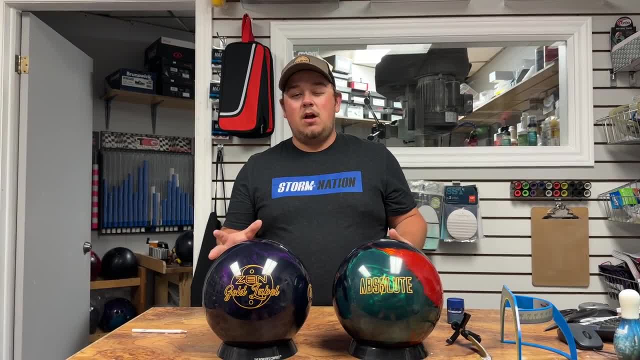 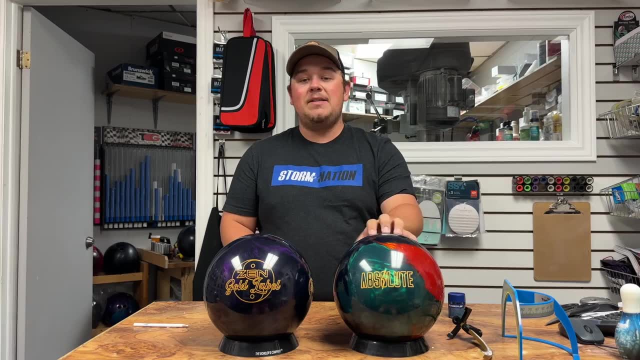 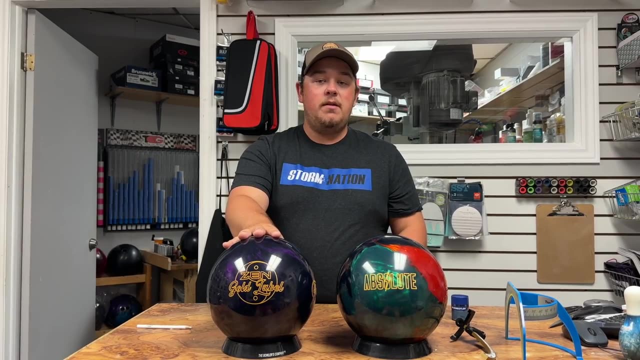 But before we get into it, let's just talk about a little bit of the reason as to why I decided this ball and this ball. This is an asymmetric ball. It's got a mass bias, It's got a pin and a center of gravity, whereas this is only a center of gravity and a pin. 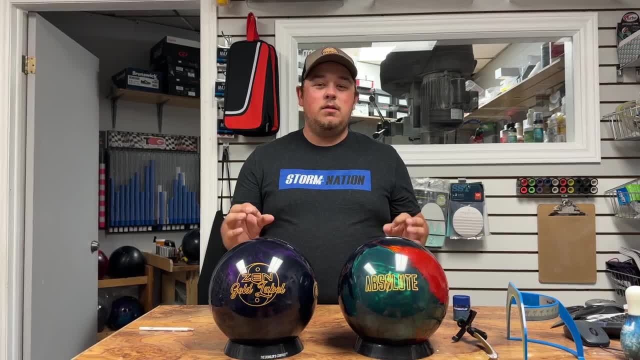 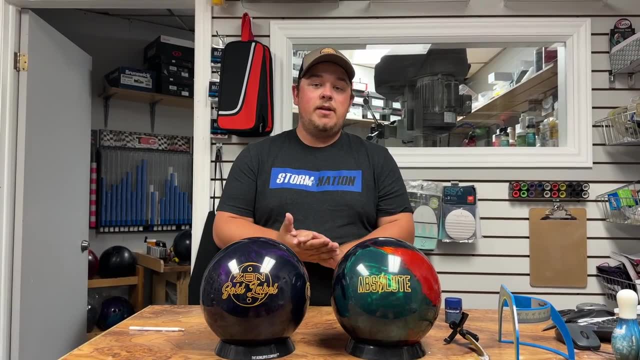 We'll come to find out. the center of gravity doesn't really matter, That little middle mark there. I'll show you what those are in just a second. But yeah, that's exactly why I picked these balls. Let's get right into a little bit more explaining. 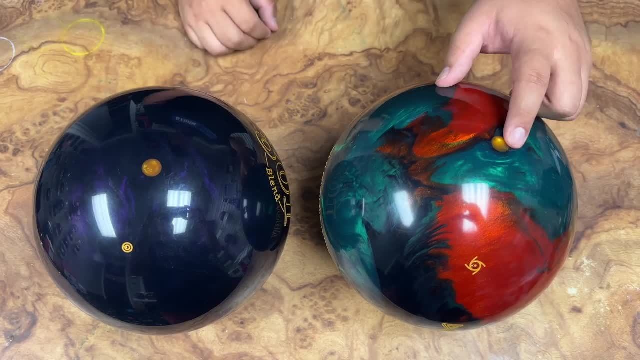 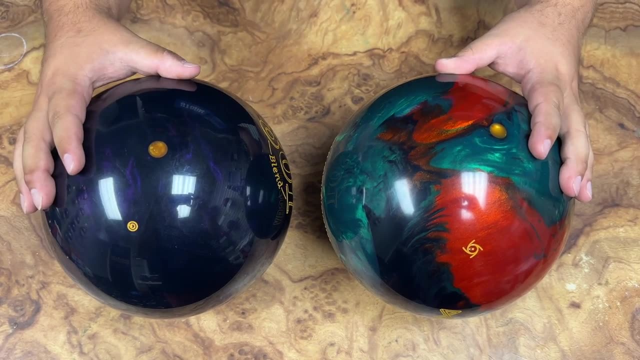 Alright, so Absolute Zen Gold Label. right here We've got the pin on both balls and then we've got the center of gravity on both balls, Obviously a little bit of a different shape, but that's just a brand thing. If you grabbed a Roto-Grip ball, it'd be a little star. 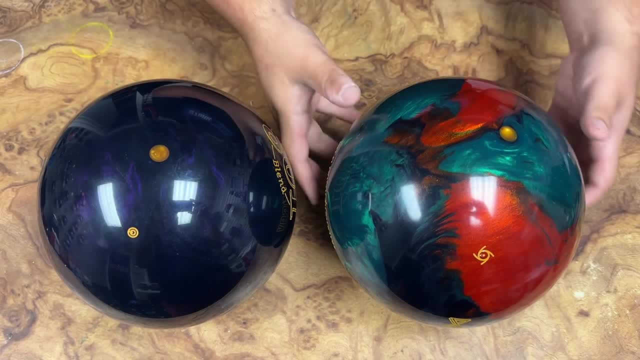 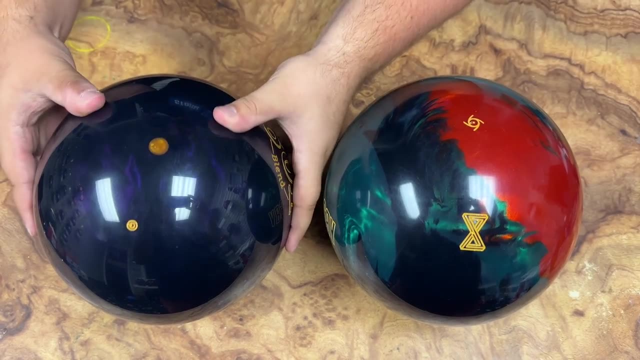 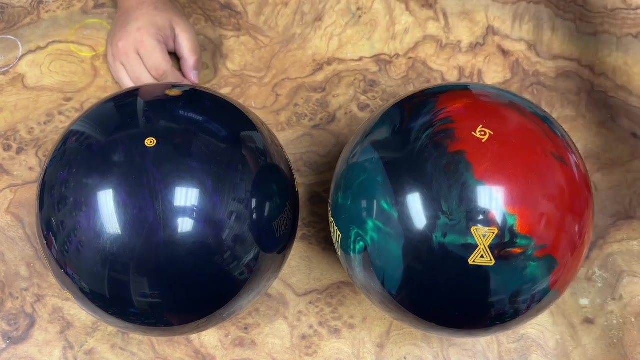 Any other brand, it'd be a little bit different as well. And then we'll flip around the Absolute here. This is your mass bias. We'll flip around the Gold Label. We do not have that mass bias. So, basically, when we start laying out these bowling balls here, we're going to use our compass here. 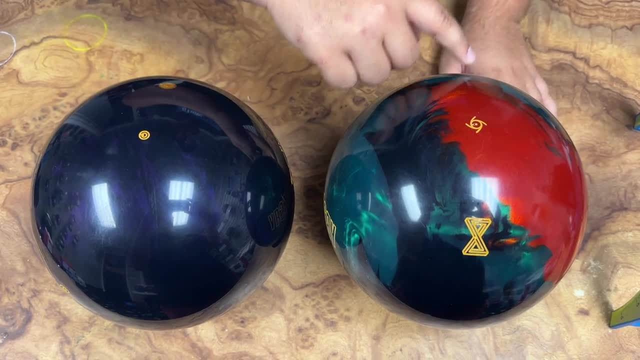 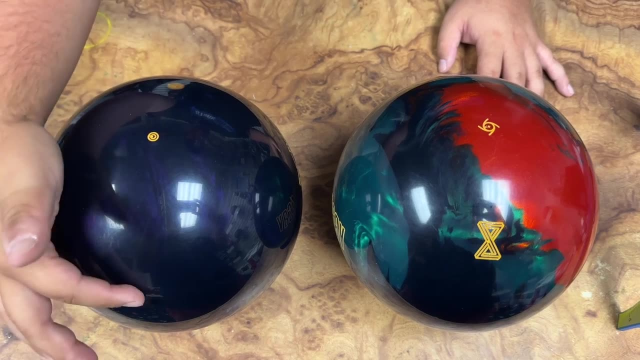 For the asymmetric ball. you draw a line straight from your pin through your mass bias and that's where you get your first two numbers there. This, the Zen Gold Label, without the mass bias, is going to be pinned straight through the center of gravity. 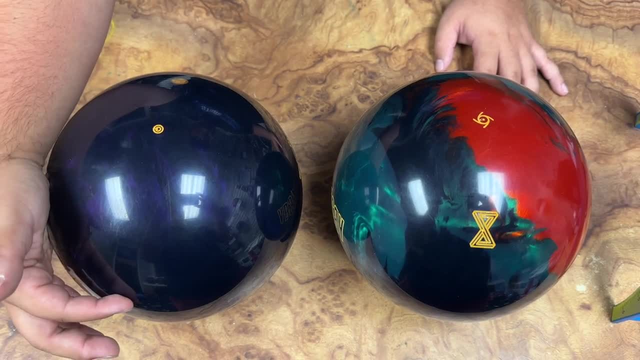 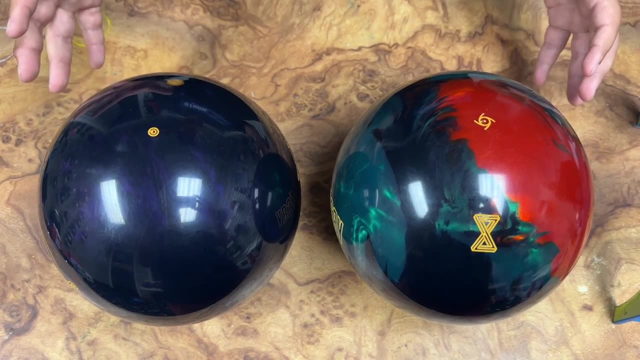 And then it's six and three quarters down on the ball here, and that's how you get that mass bias number, Because no matter what, whether you have an asymmetric or a symmetric ball, you're still going to have that mass bias measurement there. 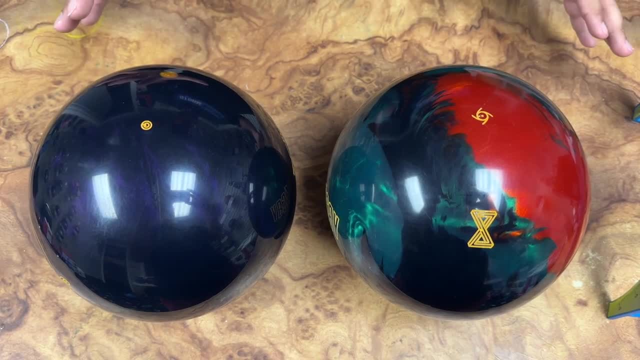 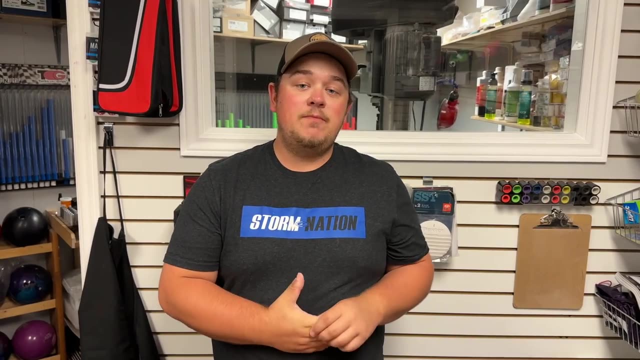 So let's get right into drawing some lines on the bowling balls and then we'll get into talking about the layout and why we picked the numbers. we did So I mentioned before we're using the Storm Vector Layout System- Three measurements here. 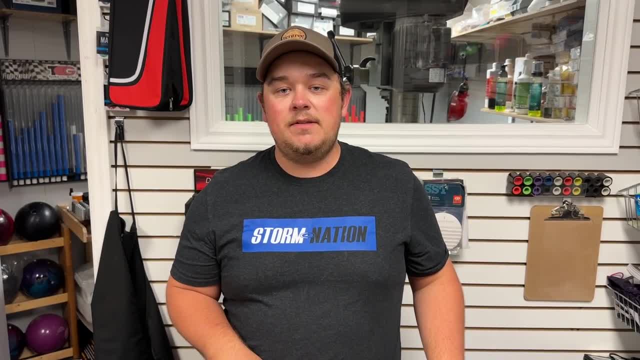 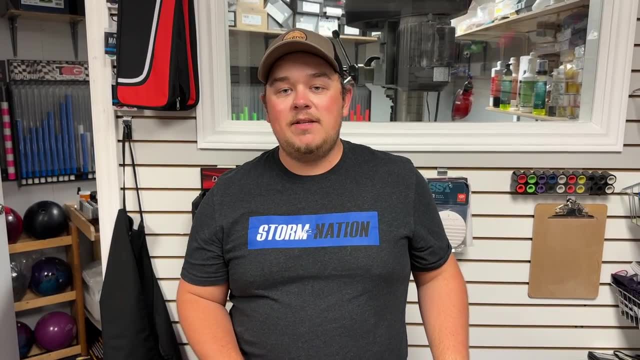 The first measurement is going to be your pin to PAP distance. So you're going to create an arc on the ball there and we'll show you that in just a minute. The second measurement is going to be your mass bias to PAP distance. 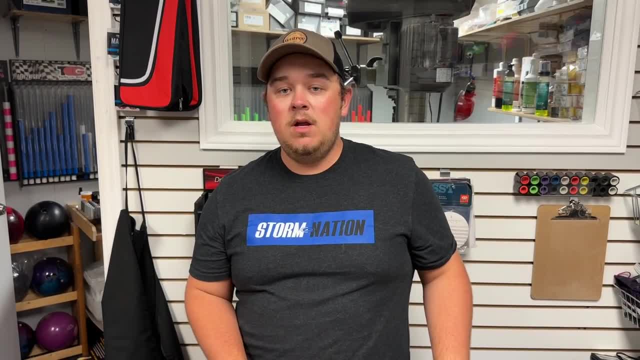 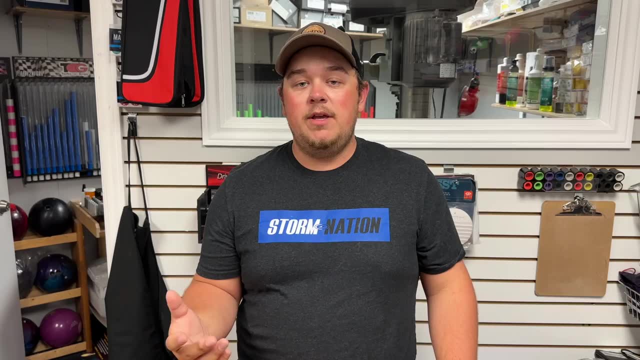 And then your third measurement is going to be your mass bias to PAP distance. And then the fourth measurement is going to be the pin buffer And honestly, there's a lot of videos out there. Storm's got a really good three part video detailed on exactly how each of those work. 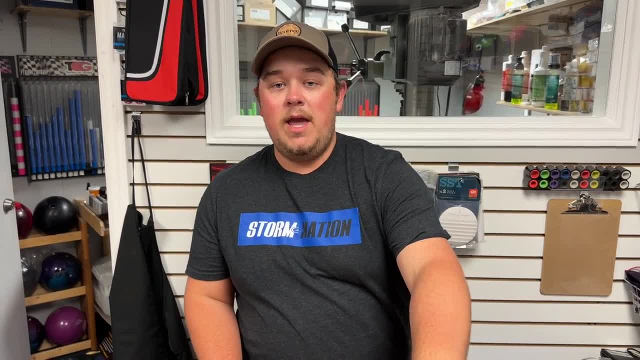 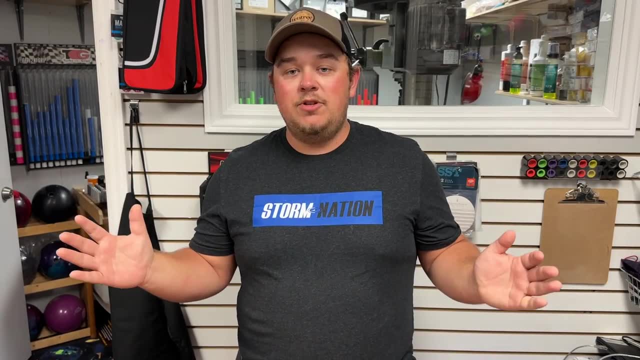 But basically, in a nutshell, the pin and the mass bias. The core is at a 45 degree angle at three and three eighths. So just out of convention, the closer you get to three and three eighths, the more unstable the core is. 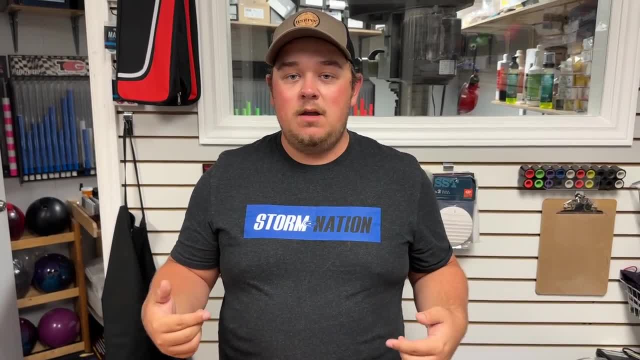 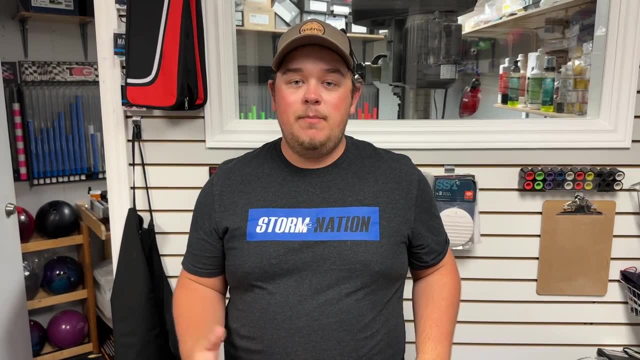 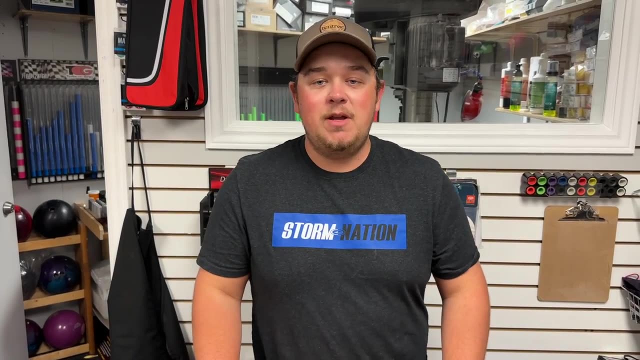 and it takes more time to get the ball stabilized around the core. so when you're a shorter pin, like a two inch pin, inch and a half pin, the ball wants to start up a little earlier. for you, if it's a five, six inch pin, even getting into six and a half inch pin, I wouldn't typically go as far. 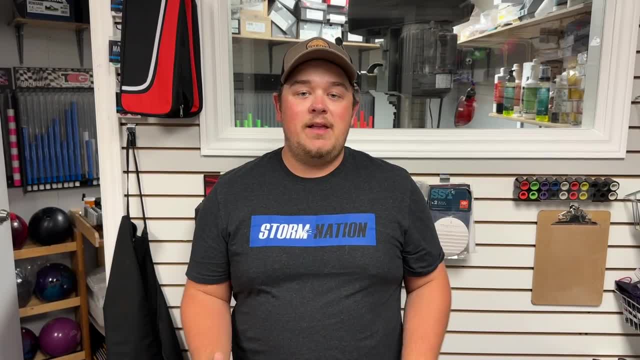 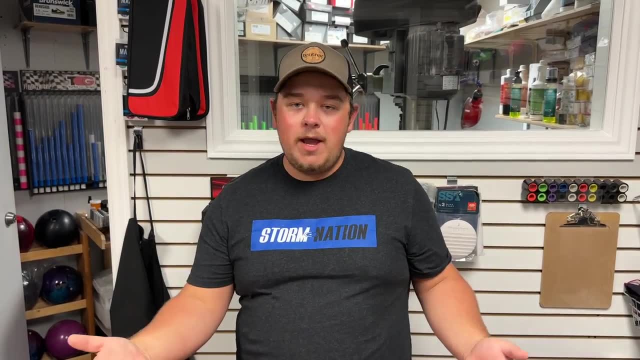 as that. I like to stick around five or five and a half, but then it's really long. not a whole lot of early roll, it's not very. it's a weaker layout. basically is what I'm trying to say, and same thing with the mass bias, the pin buffer, that 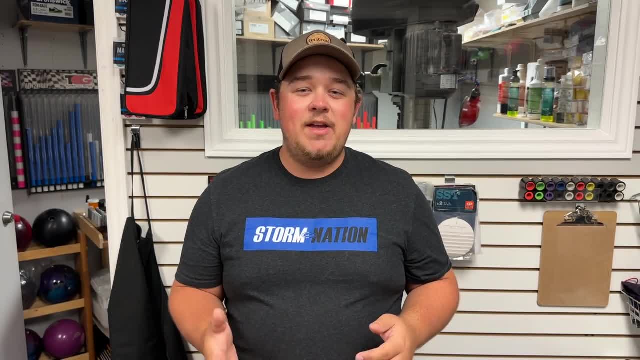 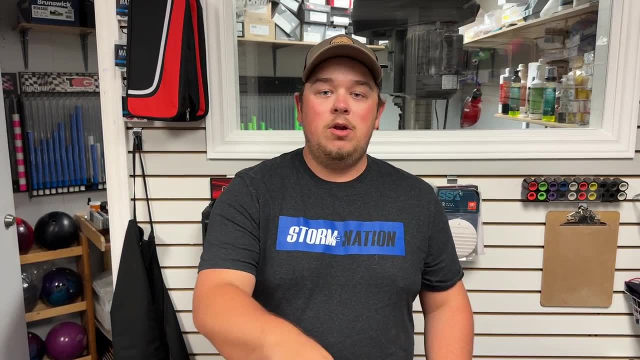 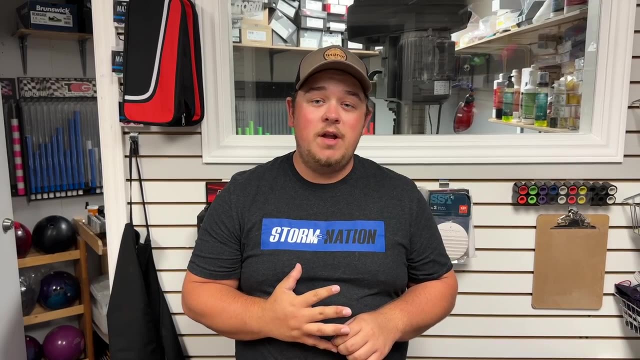 third number: typically between like a half inch and four or five, something like that, and basically that just determines where you're drilling into the ball, whether it be into the top of the core or the side of the core. basically a shorter value, like a one, two inch pin. it stores more energy. it's a. 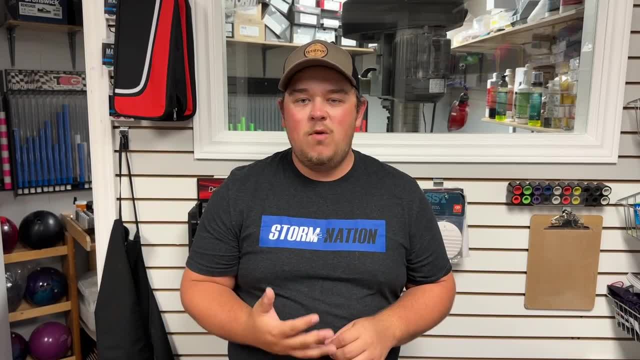 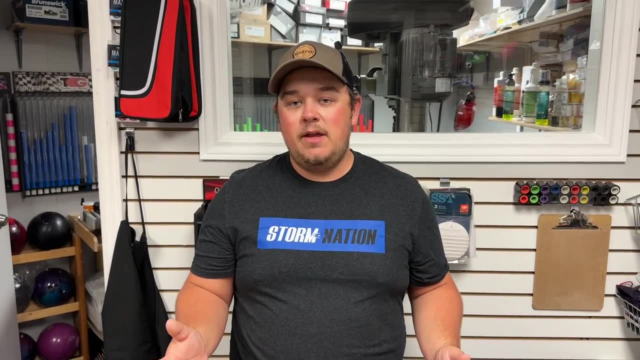 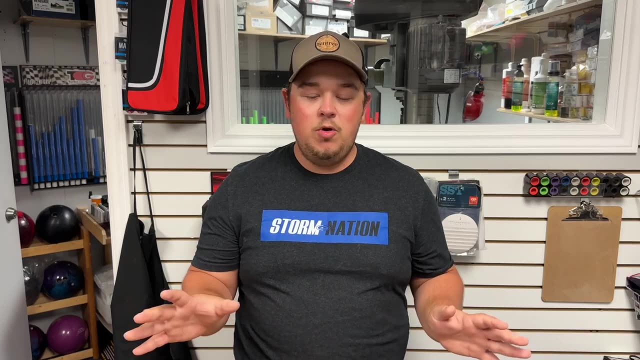 little stronger off the spot, whereas a longer value- four, five, something like that- is a little bit of a smoother transition. so now that we have a basic understanding of what numbers are what we're going to get, right into the drawing on the bowling balls, I'll do all my arcs and then we'll start talking. 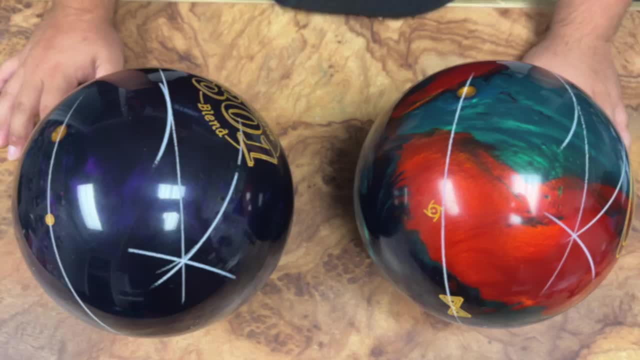 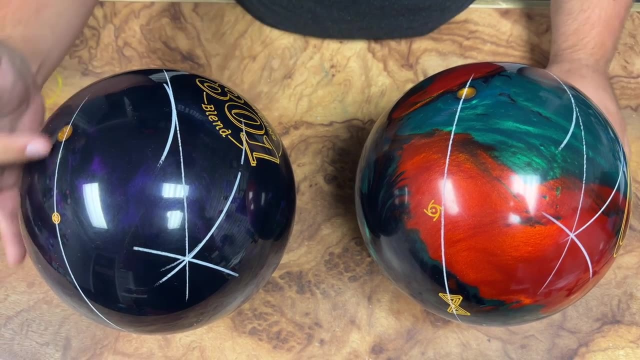 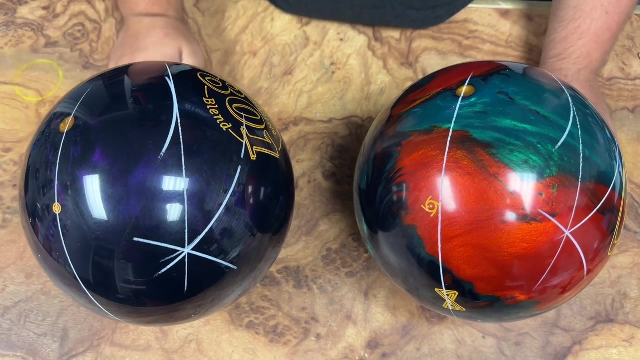 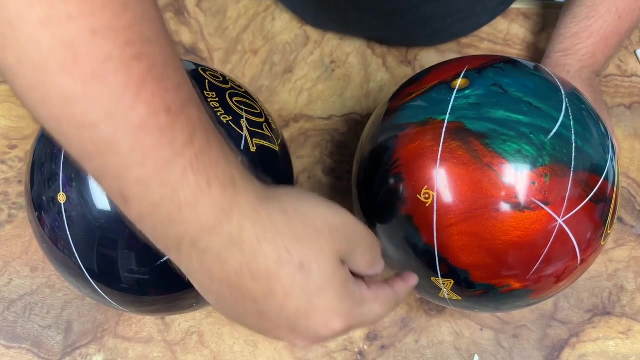 about PAP and what that means. all right, so we drew some lines on the bowling balls here, a couple different lines to talk about. so this was our center line that we drew from the pin to the mass bias, pin to mass bias here, and then from there we got our pin to PAP arc. on both we got 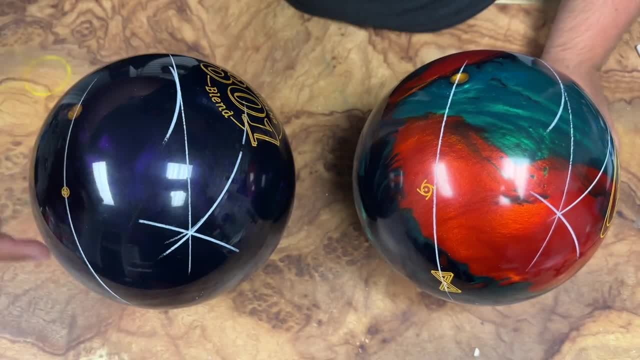 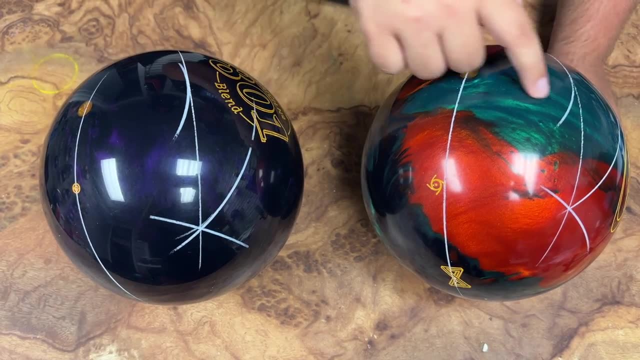 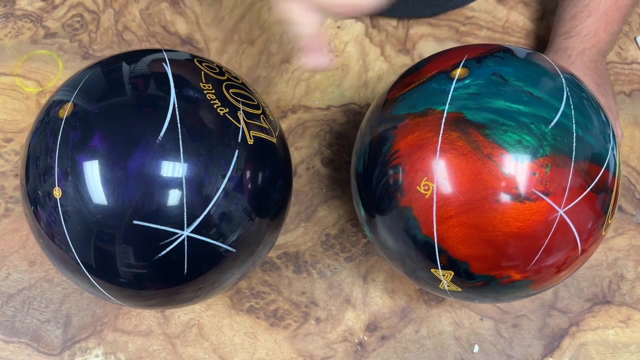 our mass bias to PAP arc on both. they're down there somewhere, right there, right there. and then we drew our pin buffer, which is just off to the side here, and then basically, you draw a straight line from the edge of your pin buffer, arc down straight through the intersection point. 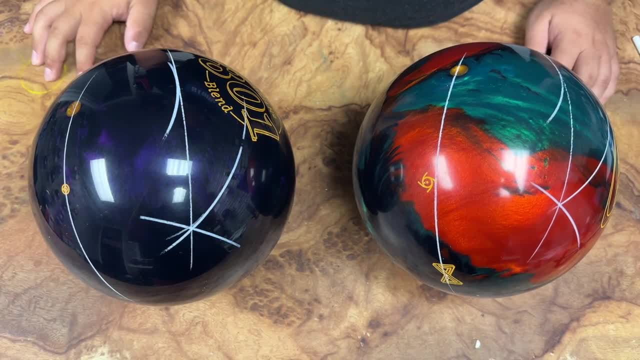 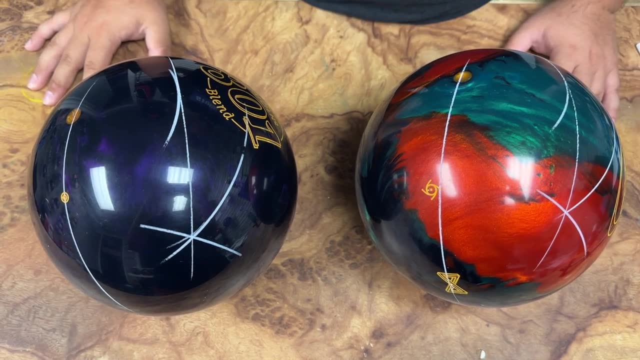 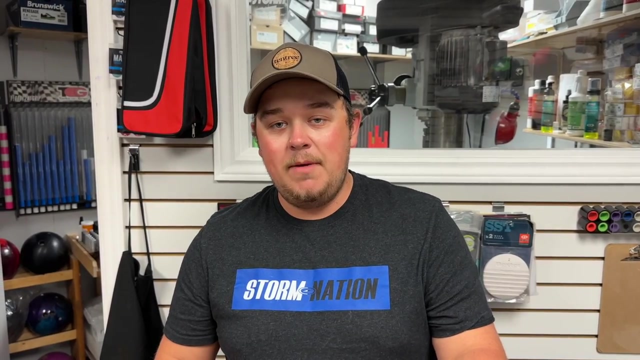 point which is right there, of your PAP, which now we get into a little bit of a more on a personal level because, like I said in the intro, everybody's PAP is a little bit different. on the absolute, I'm going to put my PAP, which is inch and a. 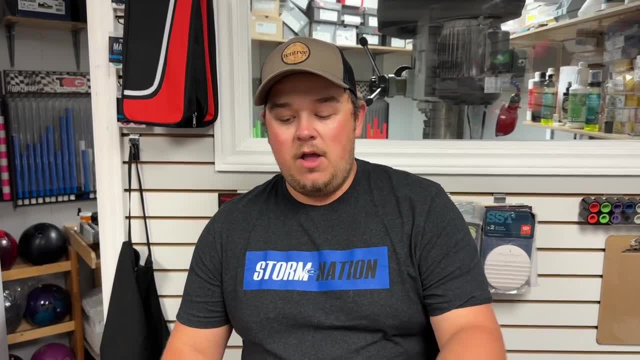 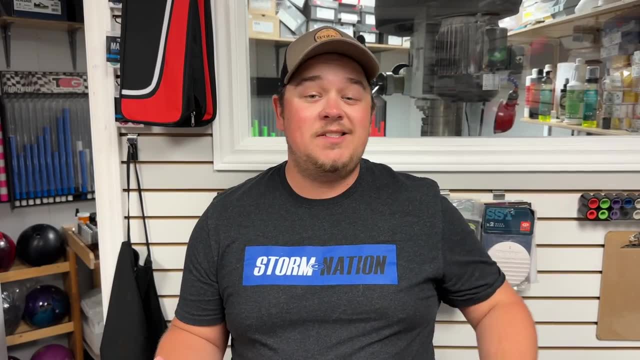 quarter up by four and seven eights over, and then on this one here we're going to put an inch and a half down by four and a half over. so you're going to get a little. you're going to see, uh, what the exact same layout looks like on two different people's bowling balls. 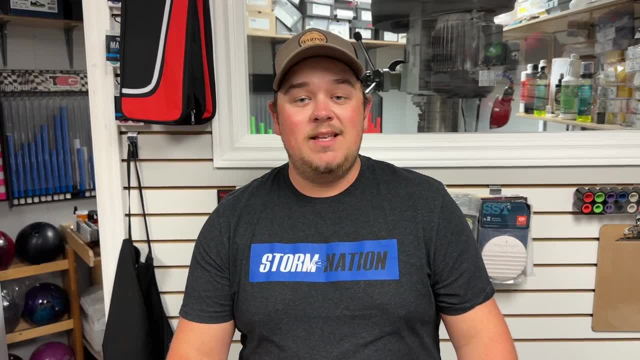 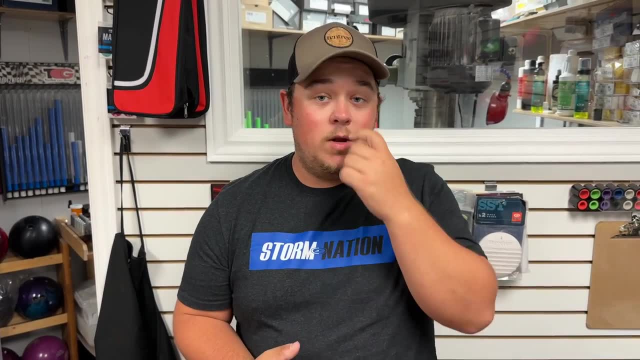 like two people could have completely different. uh, PAPs, and that's that's a really important thing to to think about. a lot of people come into a pro shop, talk to their buddies and they want to pin up bowling ball because that's what they've. 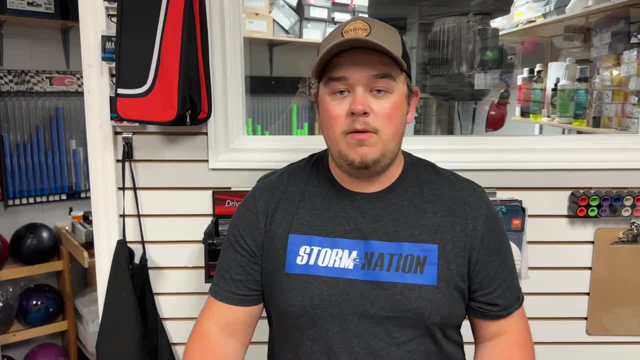 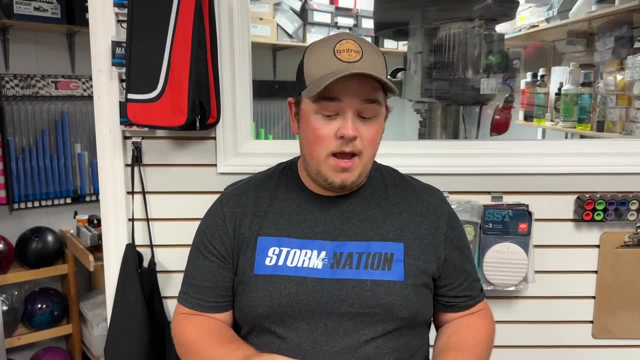 thrown in the past, that's whether they were messing around with their buddies bowling ball. they want to pin up bowling ball, but it may be completely different layout than than you think, so let's get right into that and, yeah, we're gonna uh talk about that a little bit and then we'll see the final, final result. 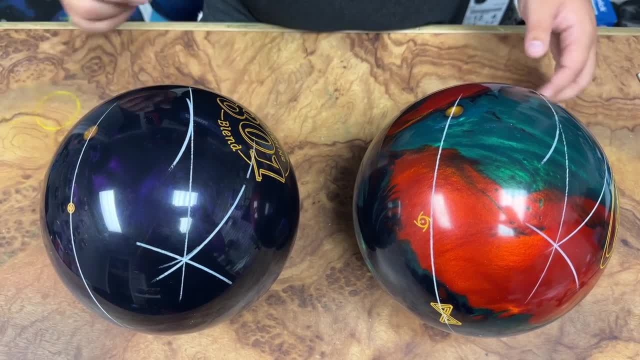 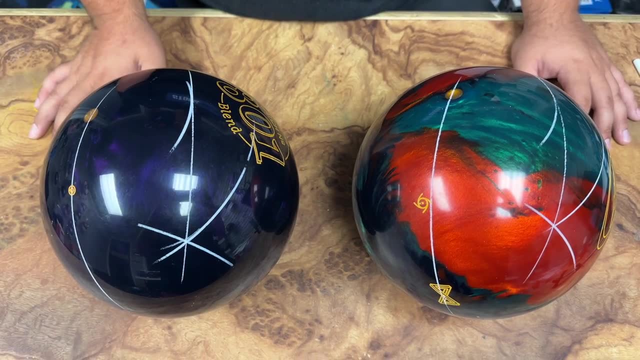 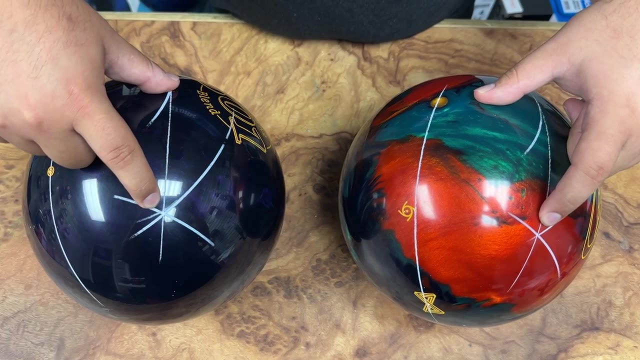 one thing I should mention before we get into uh putting the, uh the hole placements and stuff, is that, uh, first measurement on the PAP, which, on the absolute, is going to be inch and a quarter up. if this is the positive axis point right there to get inch and a quarter up, we actually have to measure down. so I guess it would be this one: we'd go inch and a quarter down. that's because that PAP, uh, if it's four and seven eighths, here we're going four and seven eighths over an inch and a quarter up. so basically, that measurement there is trying to get you back to. 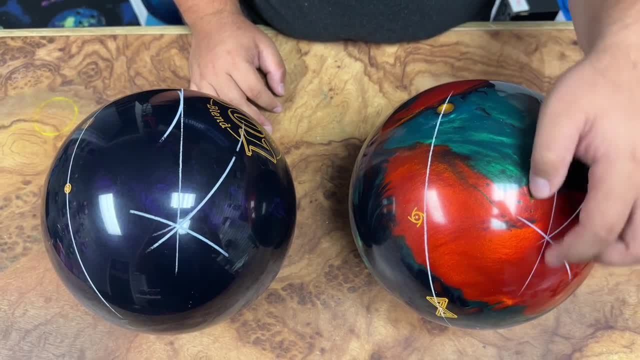 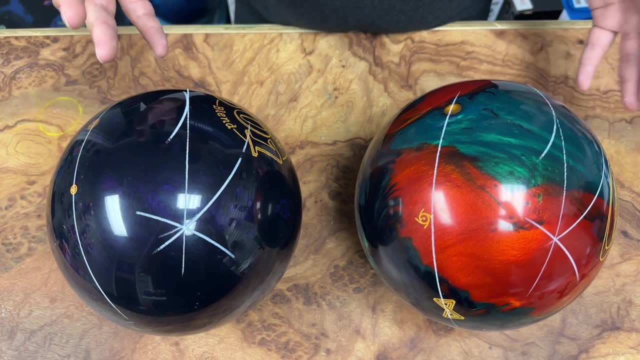 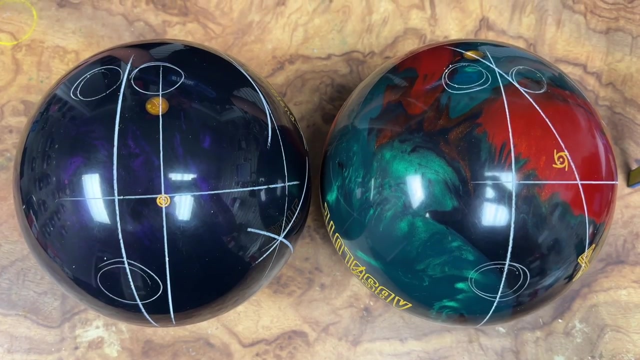 the original uh positive axis point, not your personal point, uh, so let's get into putting lines on it. we'll get the whole locations marked out and then you can see how different it is between, uh, the two uh PAPs. so, yeah, let's get right into that, all righty. so there we are. 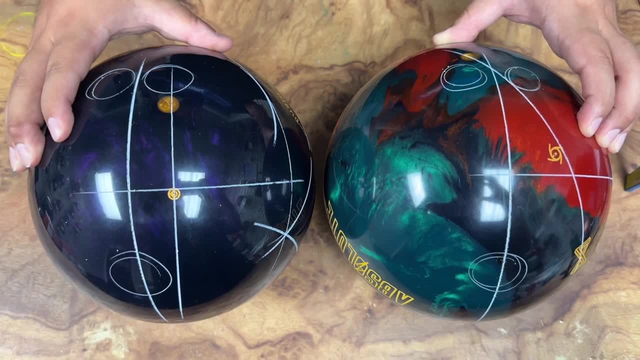 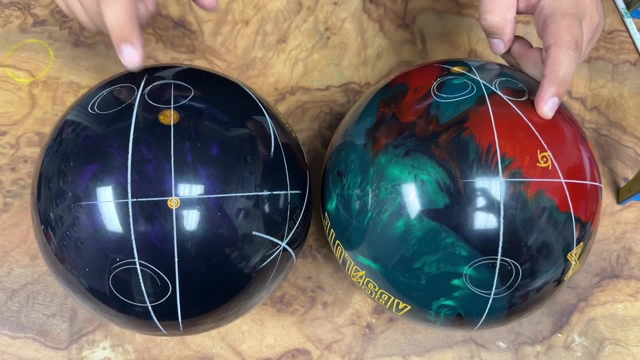 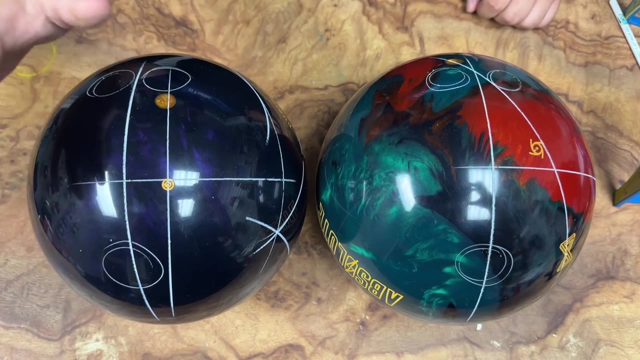 we got five by four by three and five by four by three on two different bowling balls. here, as you can see, pin pin placement completely different, and that is simply because of the PAP. like I said, on this one we are inch and a half, uh, inch and a half up and four and a half over, uh sorry, reverse. 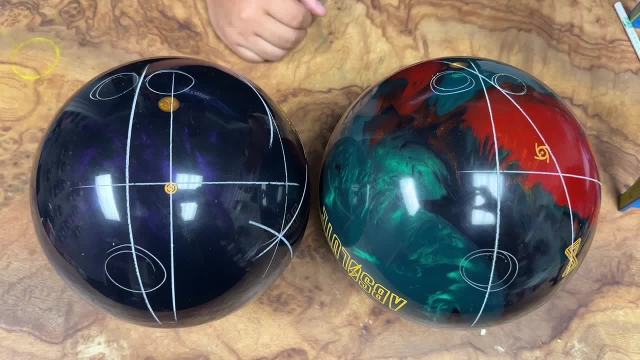 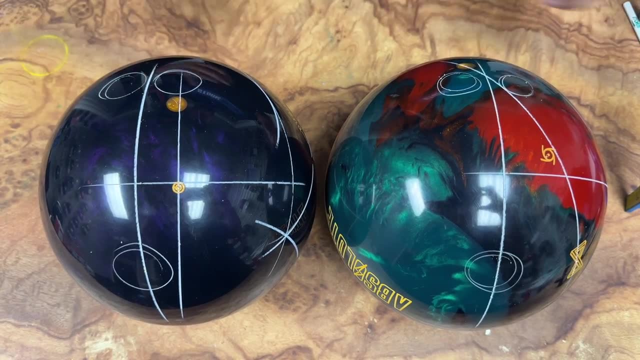 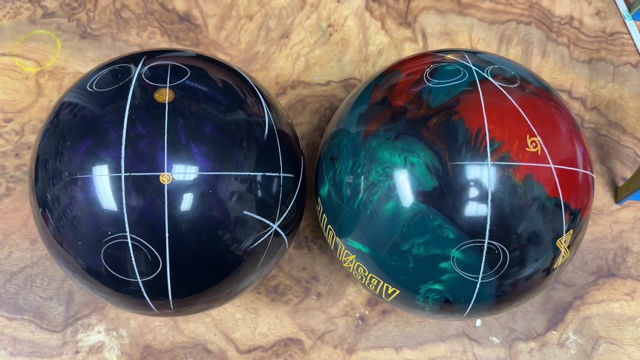 inch and a half down, four and a half over, and this one was inch and a quarter up, four and seven eighths. so that's the way. it is so simple as that. if you don't know your PAP, uh, talk to your pro shop. uh, normally that's their responsibility. anyway, it's really nice to know all your stats. 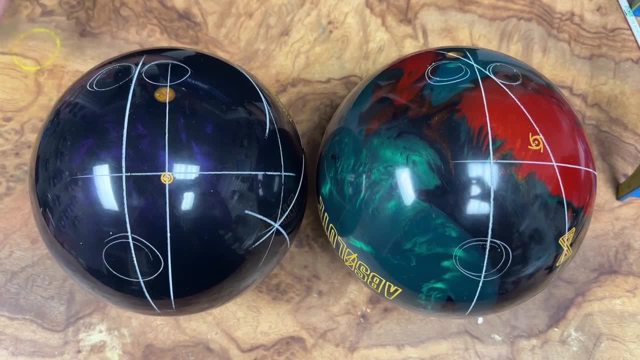 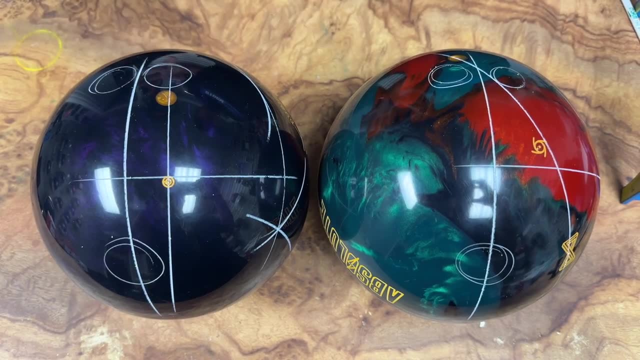 kind of what you're looking at. so if you do decide you're gonna get a bowling ball and you're not in your, in your home shop, then that's that's a good way of doing it. but yeah, this, this ball, in theory is going to make. well, obviously they're two different bowling balls, but if you had this, 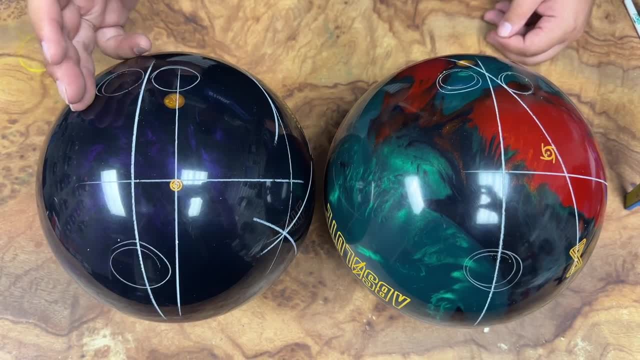 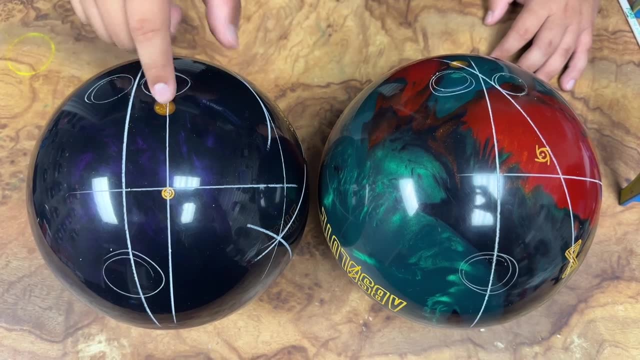 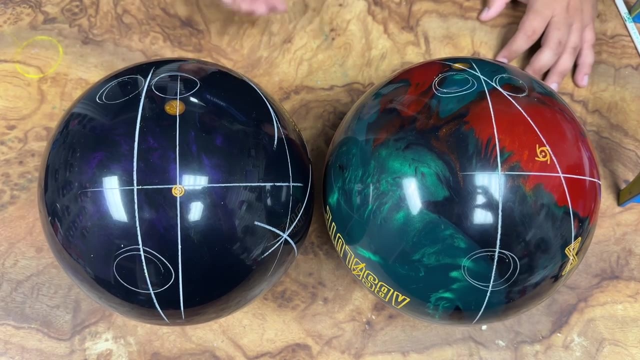 layout on this, this ball for two different people. this, theoretically, is going to be your. uh, it's going to be the same. so the five inch pin tends to be a little bit of a later uh response time. it's not going to be your most uh strong layout like a three and three-eighths one. uh, that three or, sorry, the. 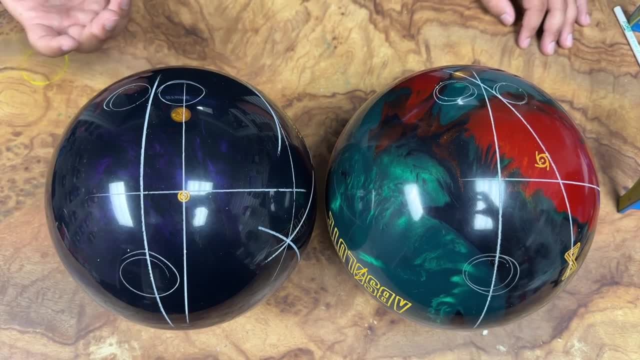 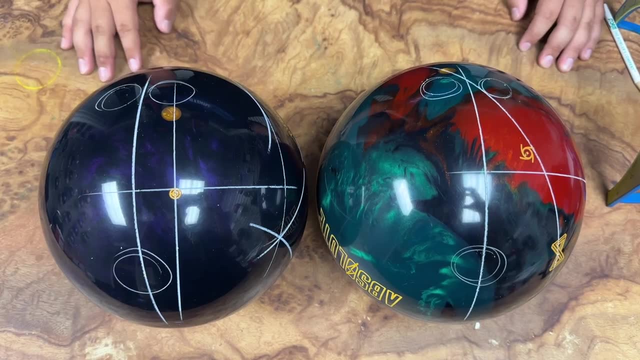 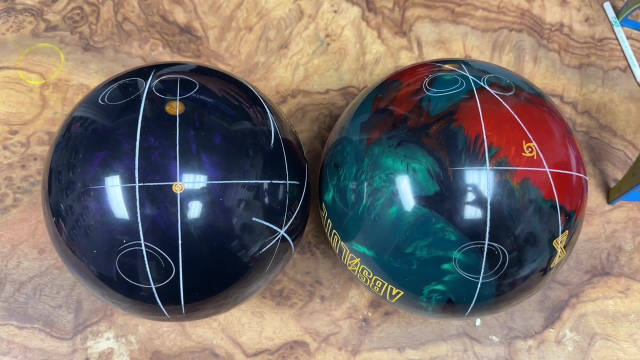 four inch uh mass bias number a little stronger and that's just going to make a transition just a little quicker. and then the three inch uh pin buffer is just, it's a pretty standard uh pin buffer. it's not too strong, not too weak. and if you had this layout for different PAPs on. 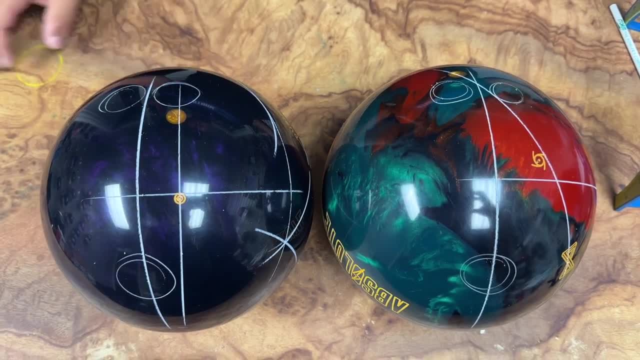 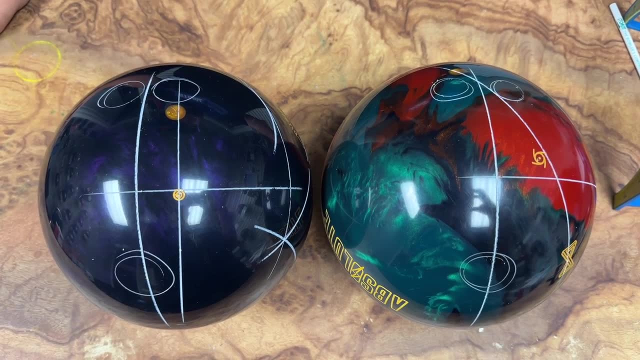 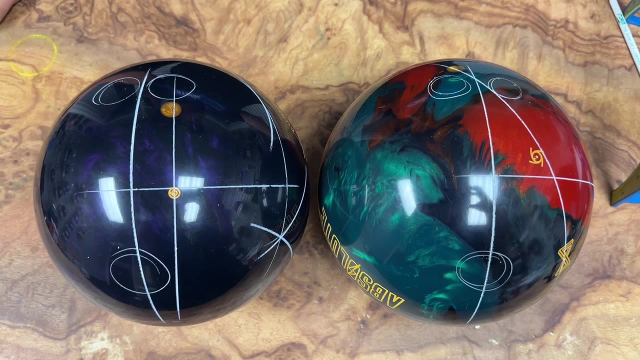 the same ball, then you would get theoretically the same thing. obviously, people throw the ball different. there's a bunch of different styles out there and it's all good. it's just about knowing what is um good for you and what is going to work the best for you. uh, let's get into. 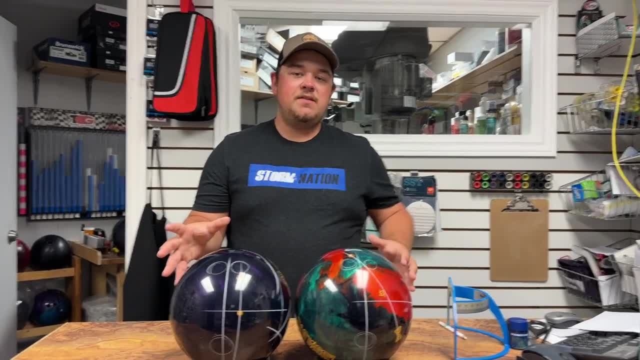 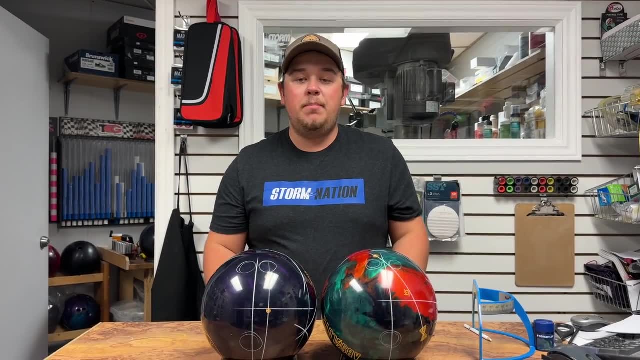 up this video. all right, guys. so that kind of wraps up today's video. uh, we're going to do a little bit of a recap, just because, uh, we talked about a lot of stuff, a lot of new things for some people, and don't want to have people confused. uh, just plain and simple, these balls have the. 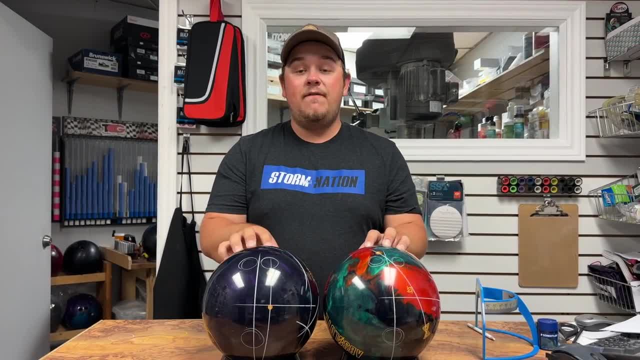 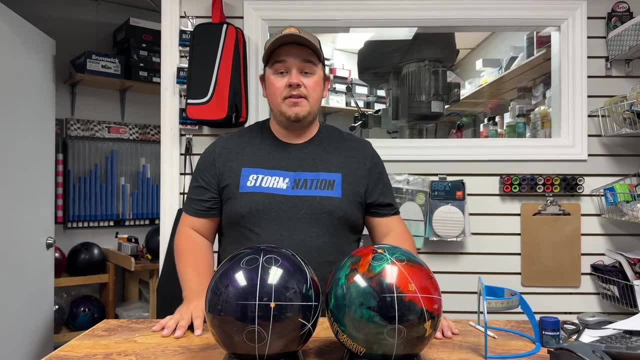 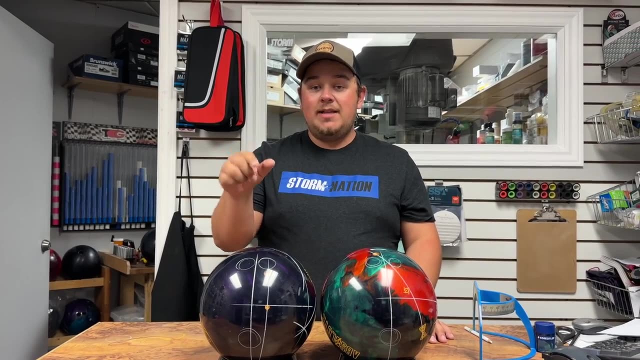 exact same layout on it, four by four, uh sorry, five by four by three. uh, different PAPs, which puts the pin in a different spot. uh, just to recap, the PAP is your positive access point. uh, that's the point in which, when you release the ball, it spins. that's, that's the access point. 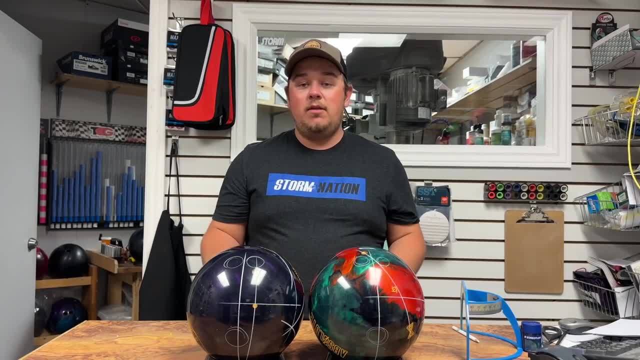 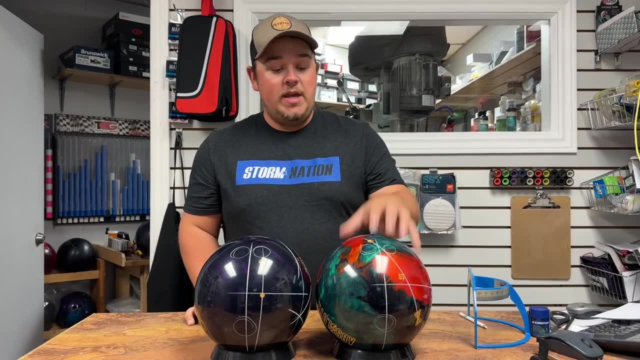 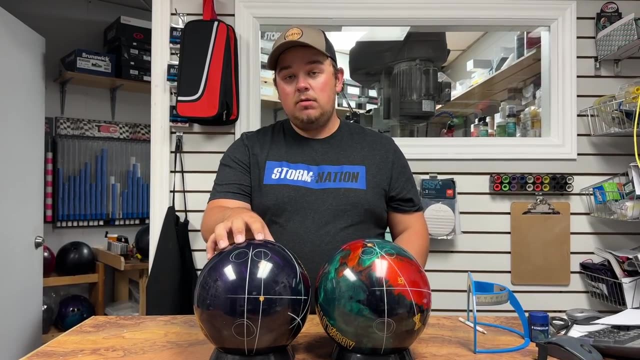 your ball is spinning at at release. obviously it migrates down lane and that will change. but that is your point, where the axis spins on. so we did a inch and a quarter up by four and seven eights over on the absolute inch and a half down by four and a half over on the um Zen Gold label. 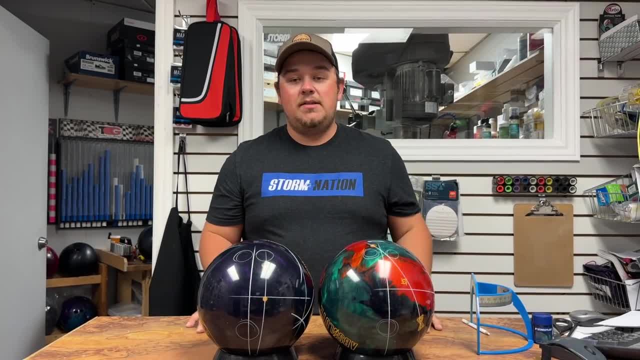 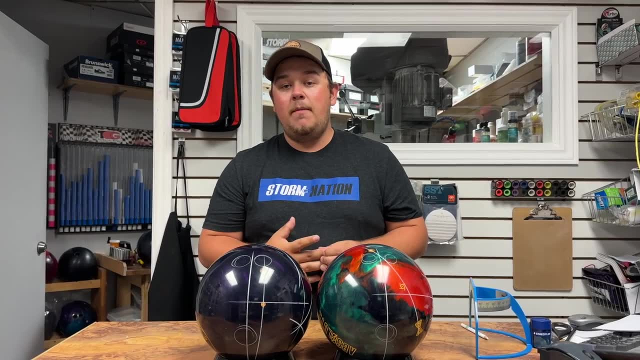 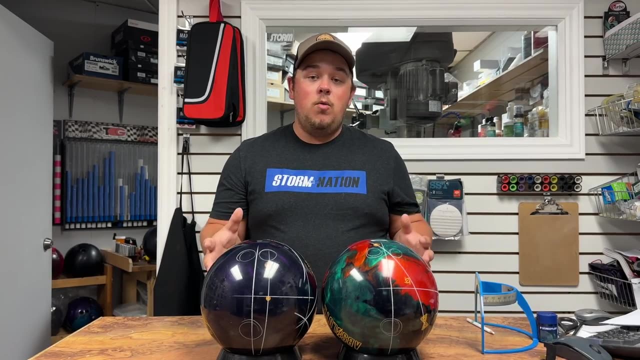 um very different uh pin placements, but they're the exact same. and that's the whole point of this video is to show you, uh, that if a pin up ball may not be a pin up ball to everybody, um, on that note, we also kind of recapped, uh what layouts do and kind of how to do the whole thing. 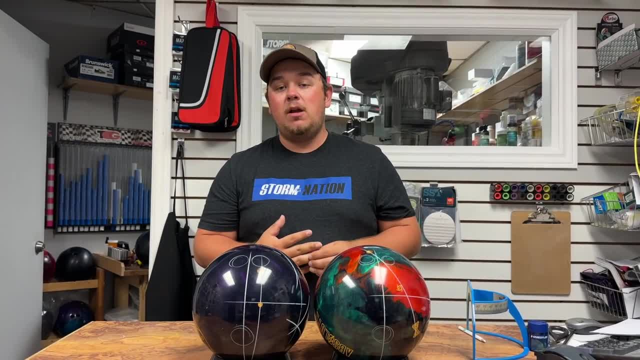 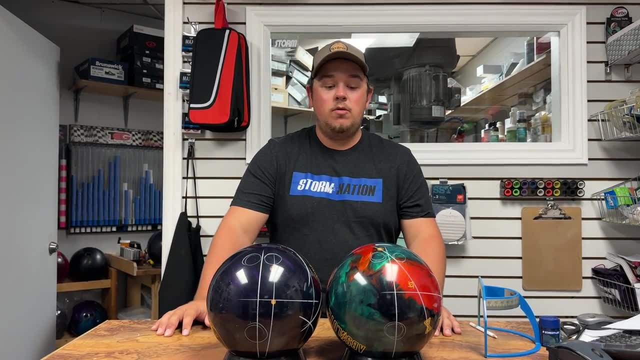 right, we, we are showing you the vector layout system. I'm probably going to come back in another video and show you the dual angle system, because this is not the only way to lay out a bowling ball, it's not the only way to do this. so, uh, on that note, we're going to end the video, uh, like, and. 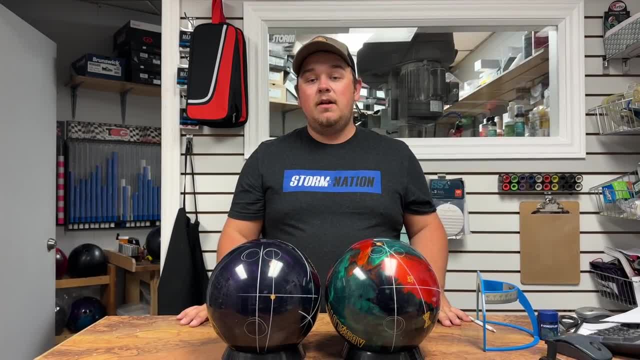 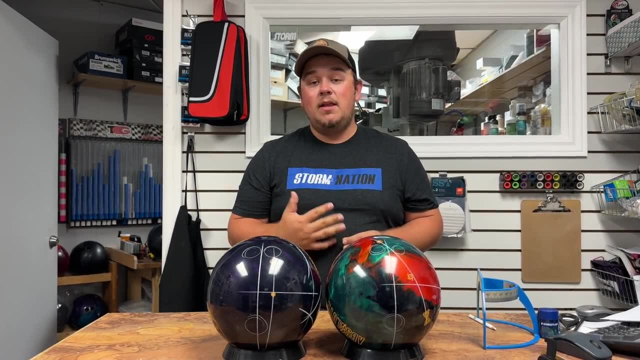 subscribe comment. uh, keep showing me all the feedback, because we're doing really well and I want to keep doing these videos and I want to keep doing the reviews and all that stuff. so, uh, like I said, like uh, subscribe comment, uh, bowl up a storm and we'll see you in the next one. foreign.